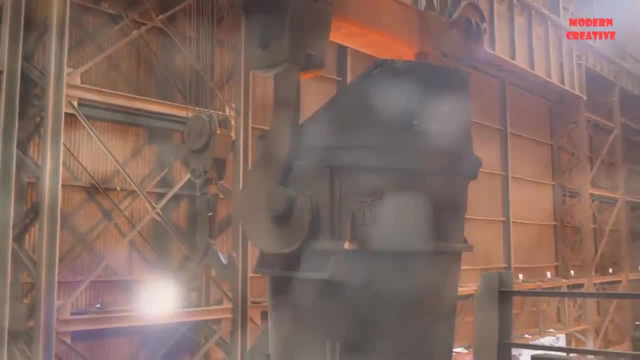 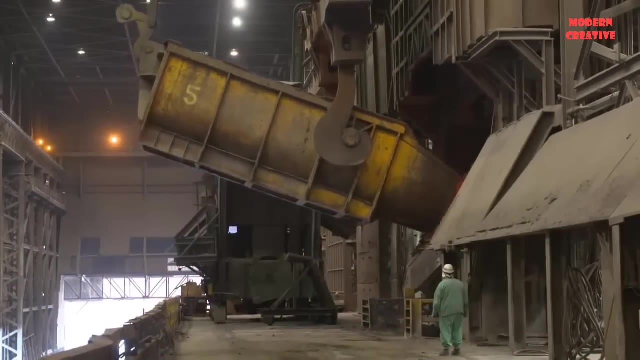 More than half the world's steel is produced in the basic oxygen process. The basic oxygen furnace is a refractory-lined tiltable converter into which a vertically movable water-cooled lance is inserted to blow oxygen through nozzles at supersonic velocity. 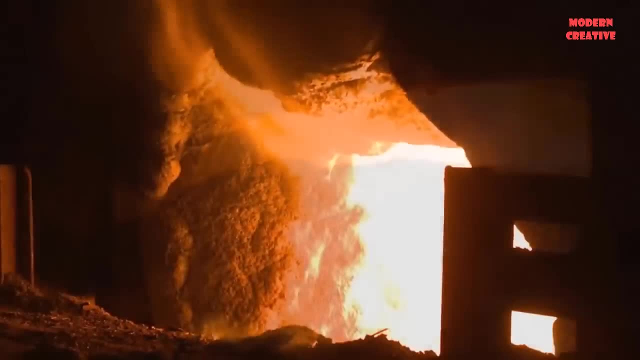 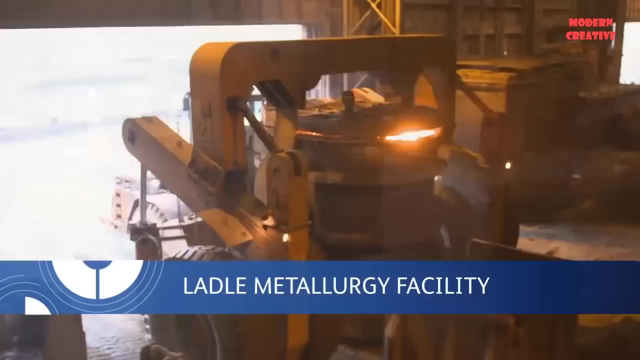 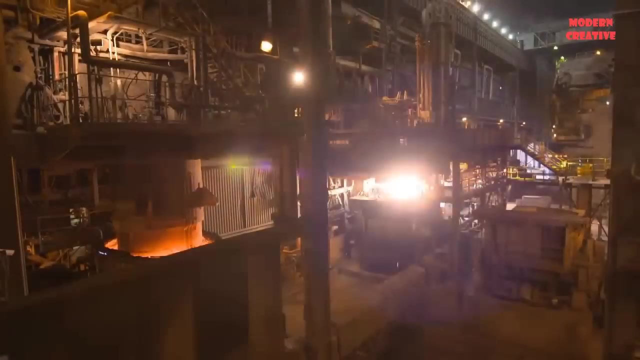 onto the charge. The use of pure oxygen at high flow rates results in such fast oxidation of the elements contained in blast furnace iron that only about 20 minutes are required per heat. IE to refine one charge. Converters vary in size and are operated for heats ranging from 30 to 360 tons. 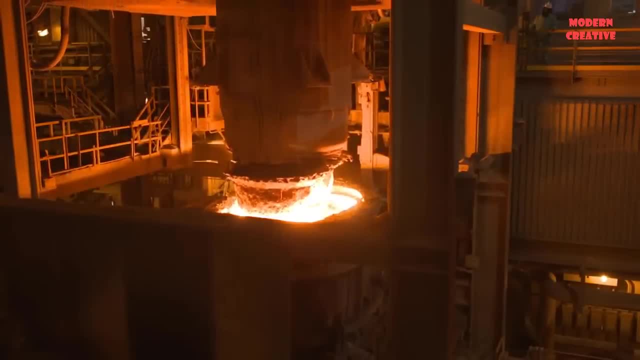 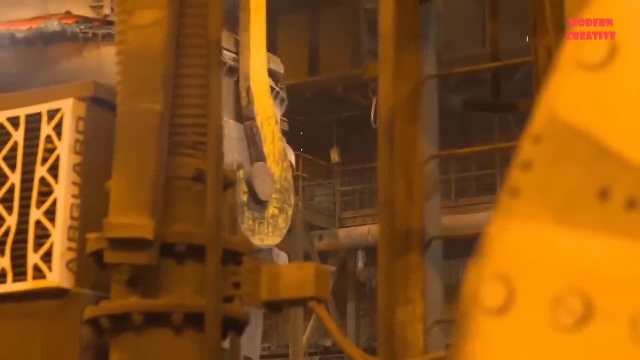 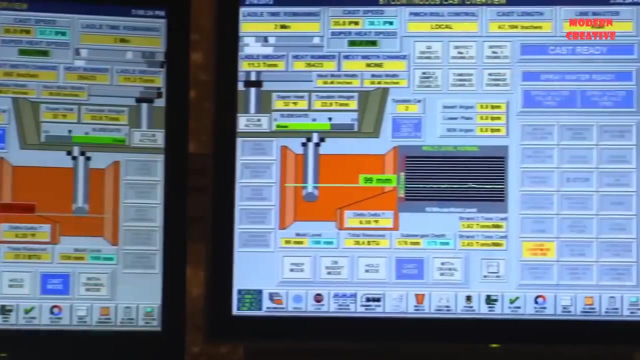 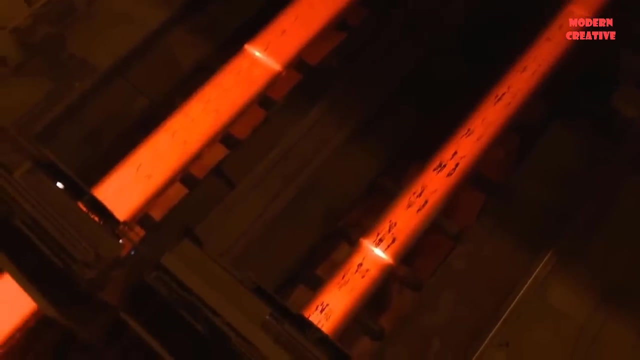 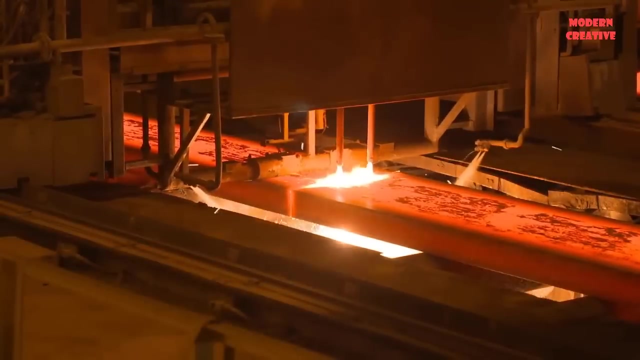 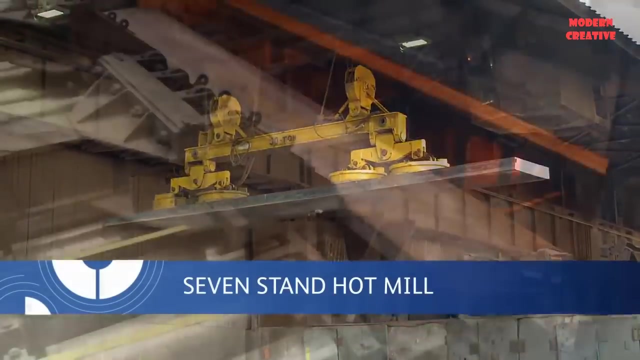 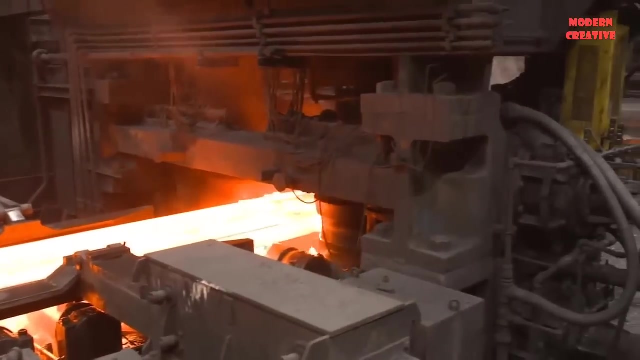 Now it's your turn to check out some我要 uj. Severstal Dearborn, 68 Inches Hot Strip Mill has an annual throughput of 3.8 million tons, 3.5 million metric tons. The hot strip mill can roll to a minimum gauge of 0.050 in. 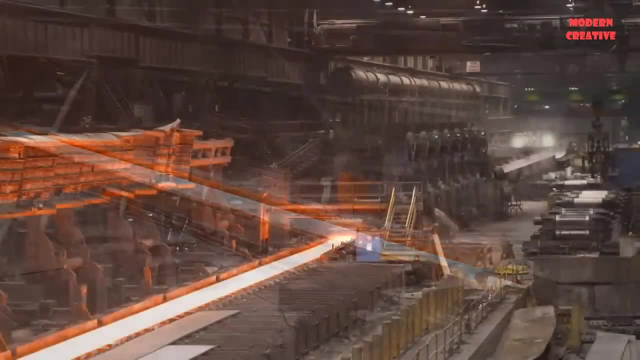 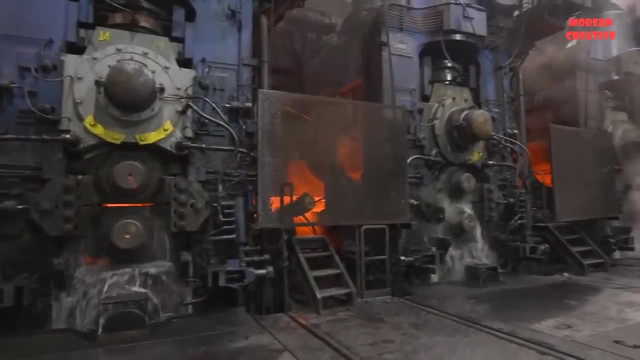 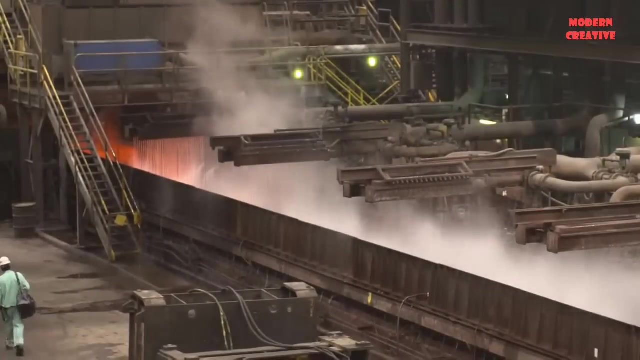 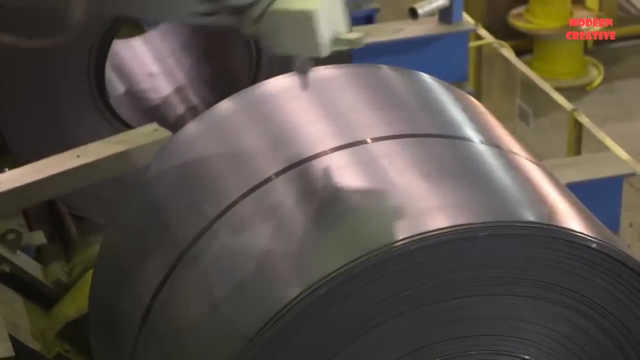 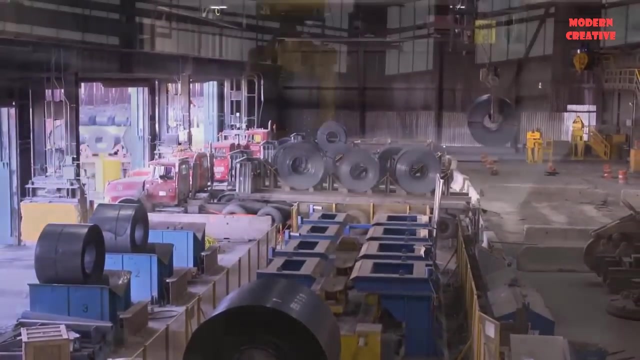 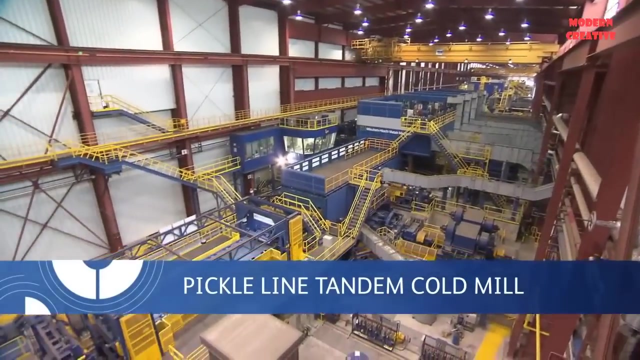 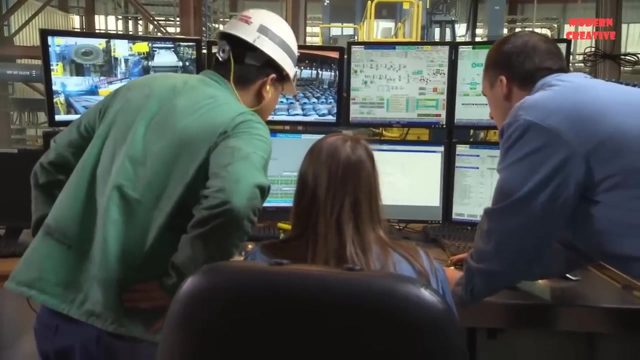 Through 525 inches, 1.27 millimeters through 13.30 millimeters. in widths from 30 inches to 61 inches, 762 millimeters to 1549 millimeters. Severstal Dearborn Cold Rolled Steel is available in thicknesses from 0.014 inches to 0.110 inches, 0.36 millimeters to 2.79 millimeters. 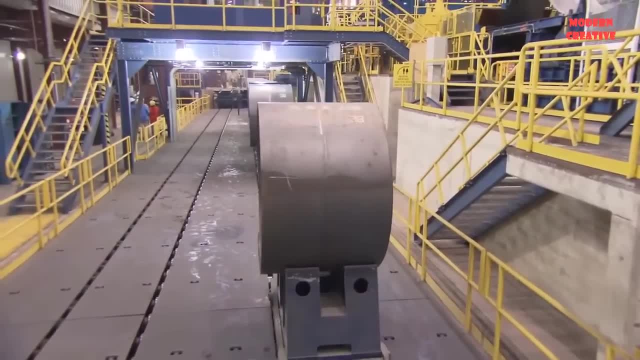 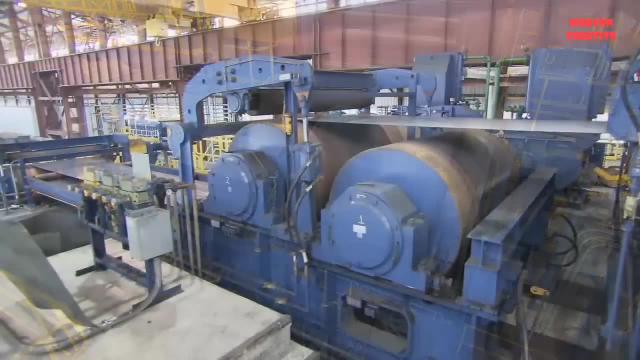 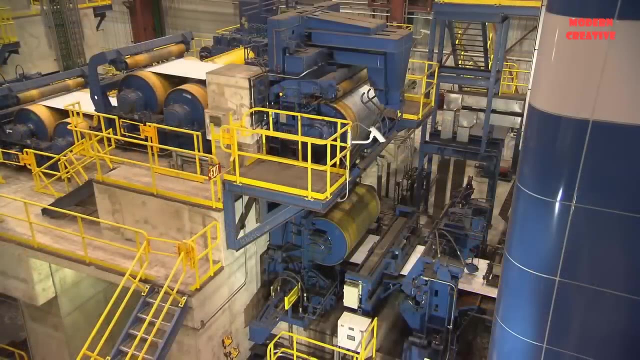 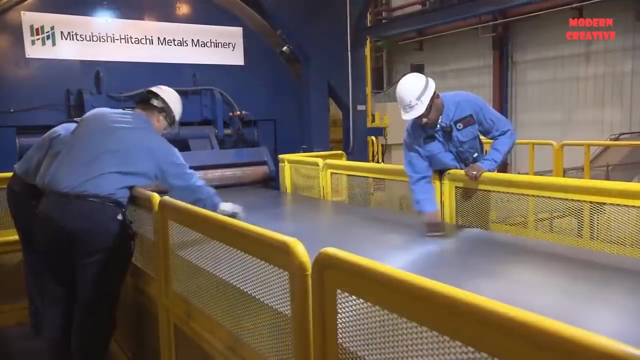 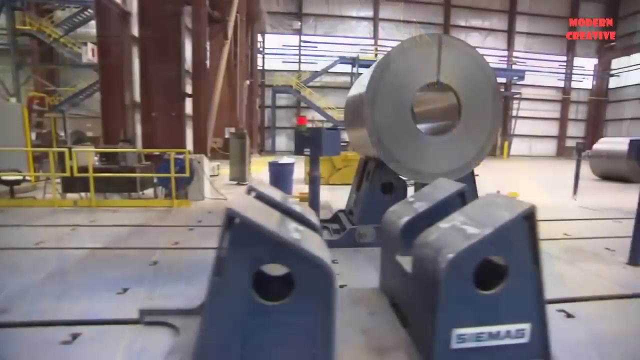 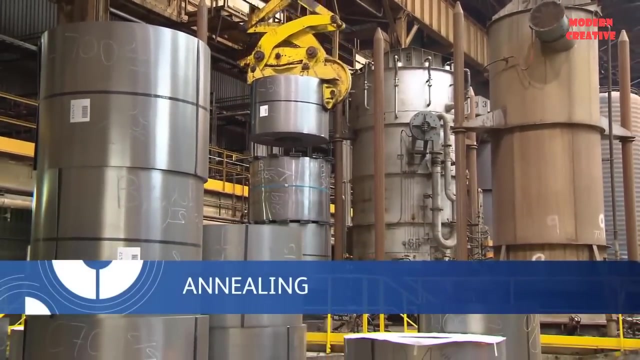 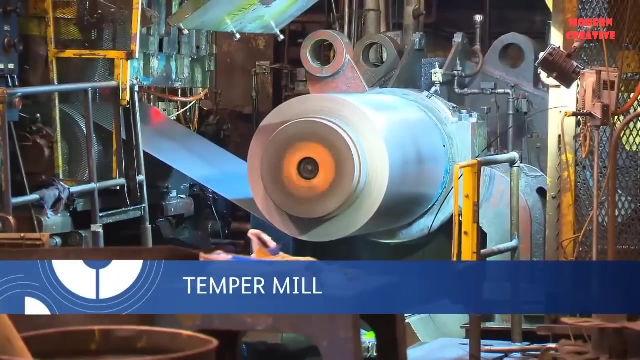 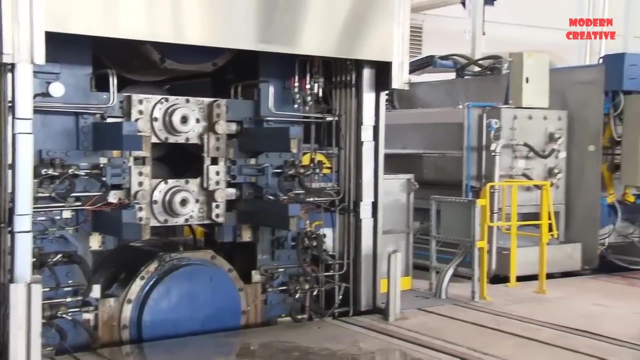 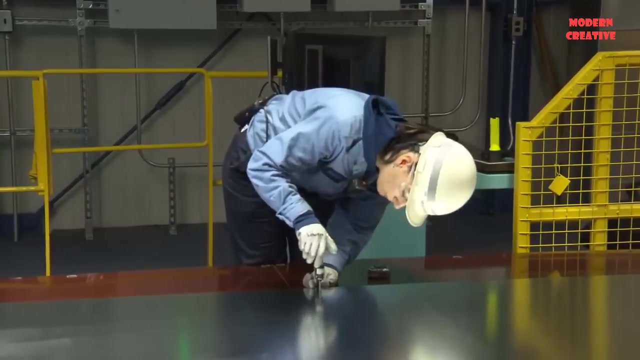 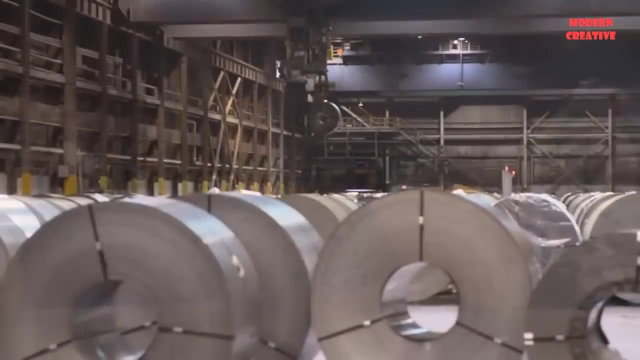 and widths from 28 inches to 61 inches, 711 millimeters to 1549 millimeters. Cold rolled steel output is about 1.8 million tons- 8 million tons a year- One big. After the production of steel coils is completed, they will be transported to manufacturing plants that use steel coils as input. 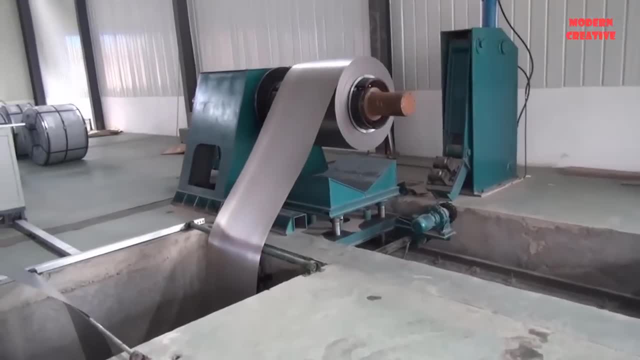 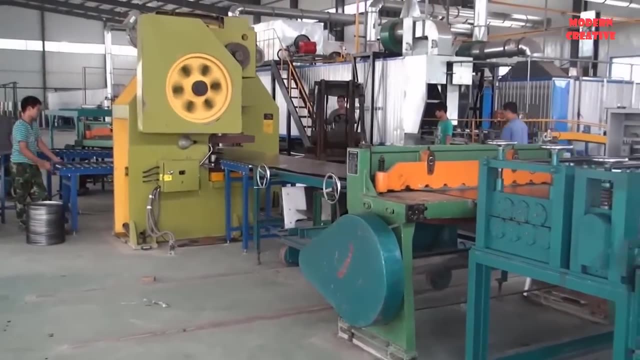 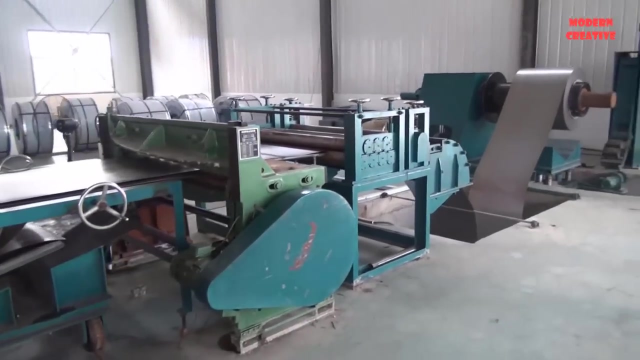 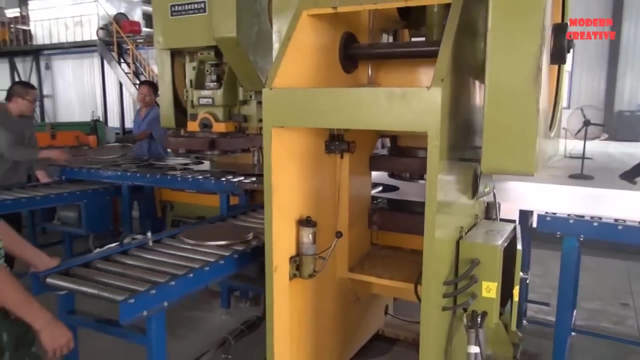 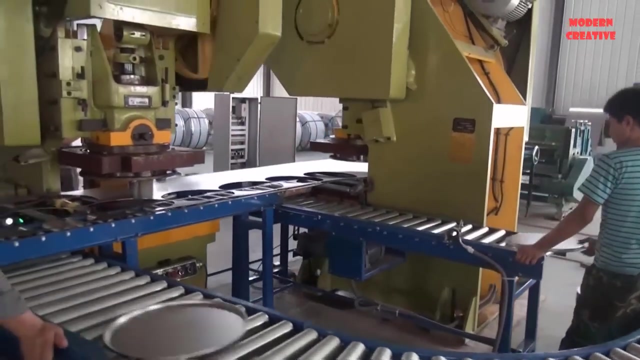 materials. In this video we will visit a steel drum production sites. To those who will visit, don't forget to subscribe and press the bell. Steel coils are fed into automatic lines and cut into round shapes to produce steel drum lids. The line is applied, the most modern technology, to help cut the maximum piece of round shaped steel from available steel coil size. 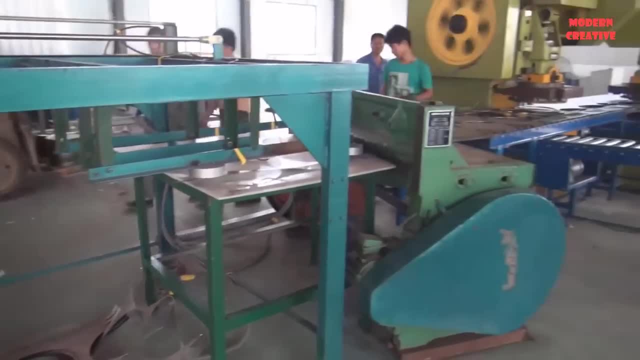 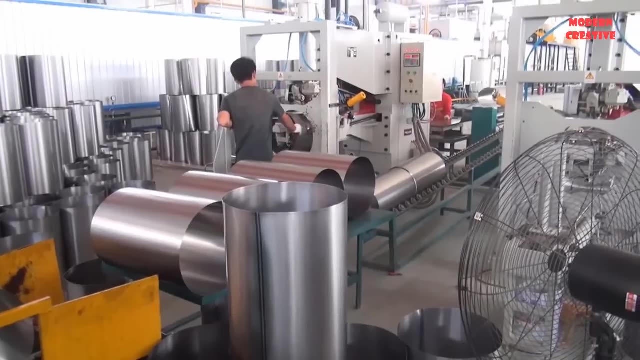 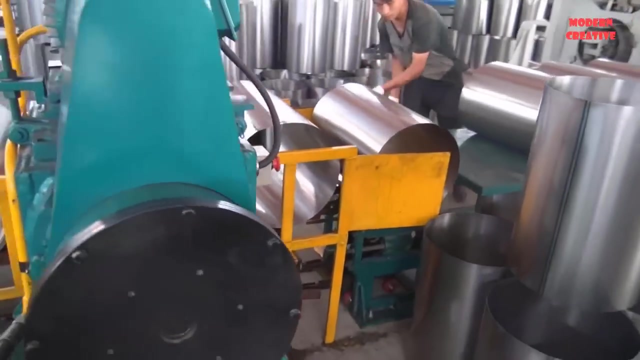 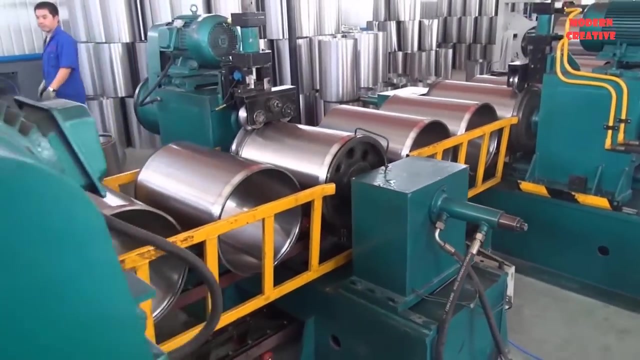 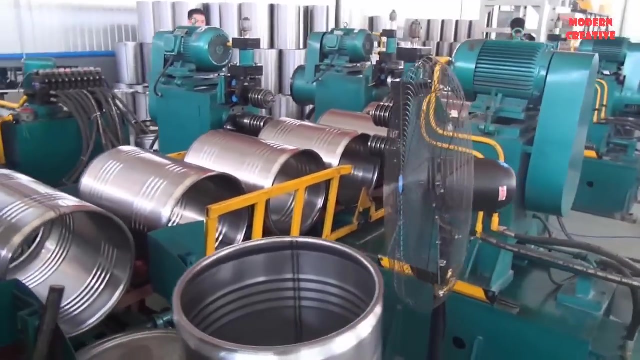 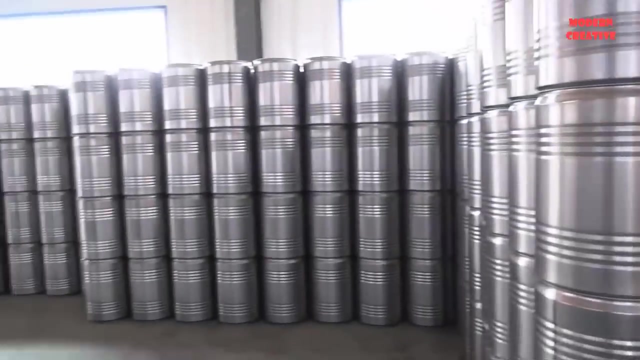 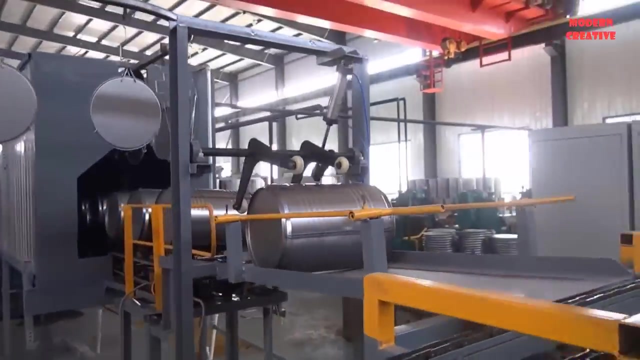 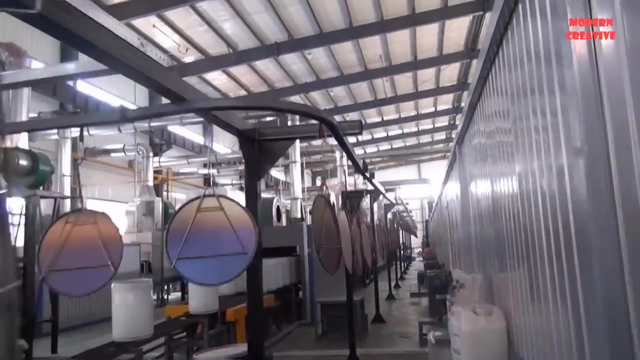 Next is to cut and bend the steel drum body, then weld the corrugated iron edges together. The front and rear of the handrails are molded to show the forward shape. The front and rear of the body are molded to show the return shape. 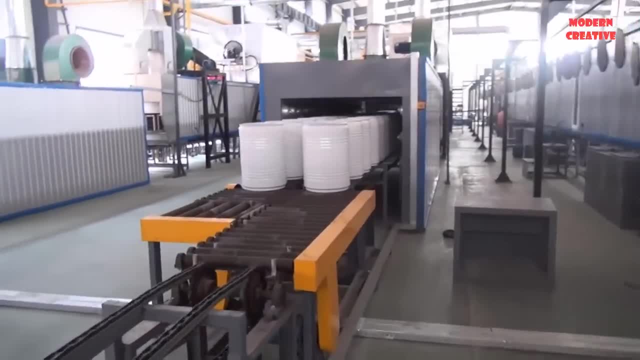 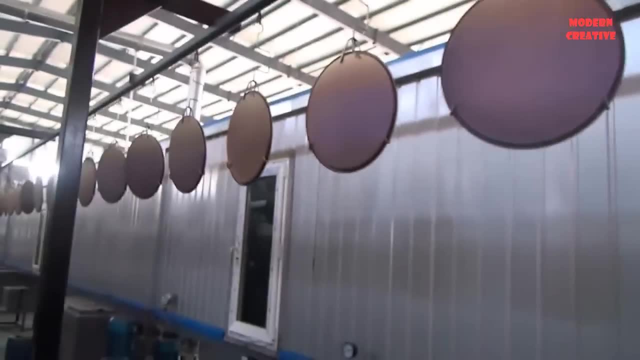 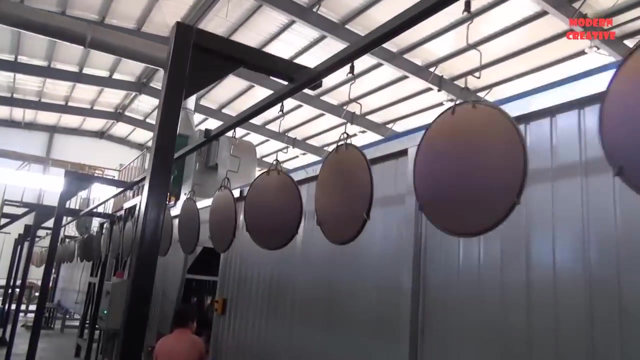 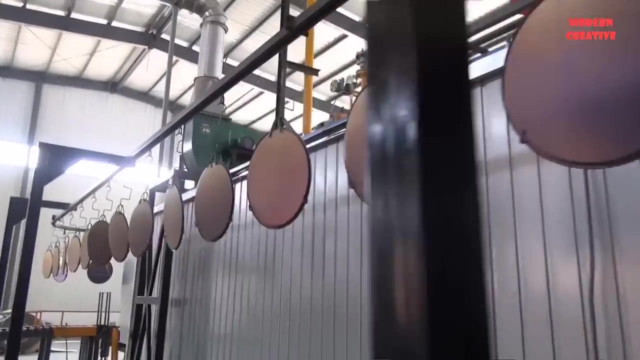 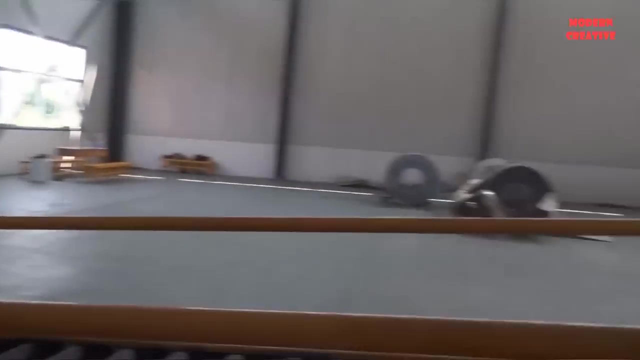 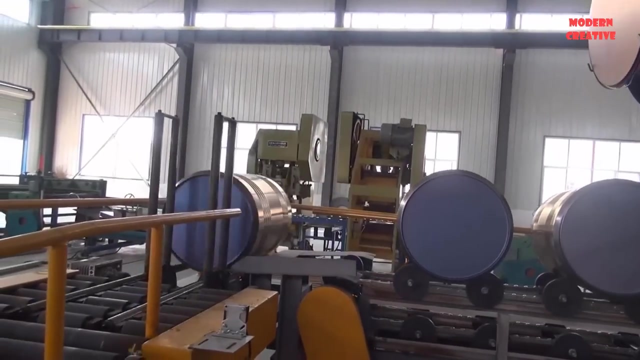 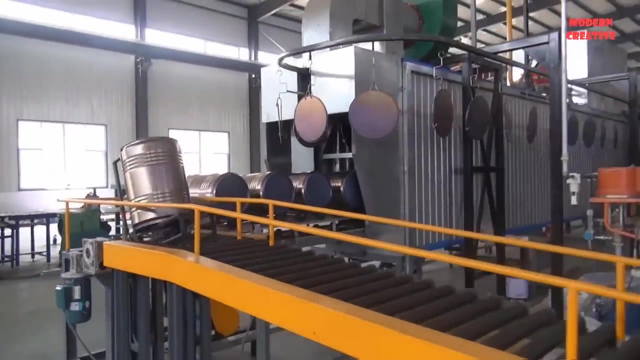 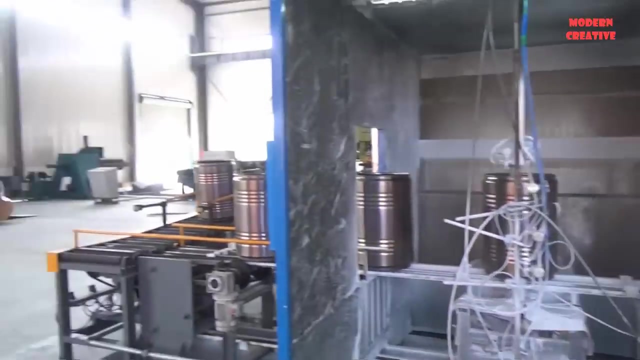 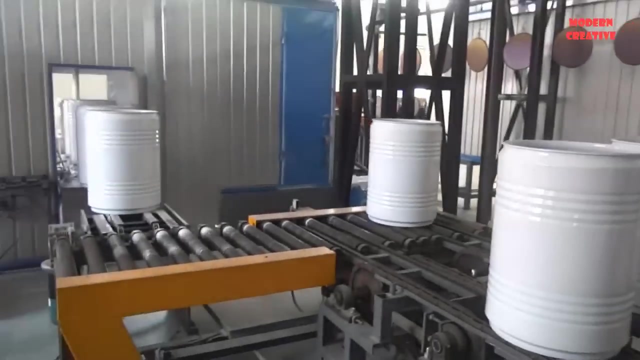 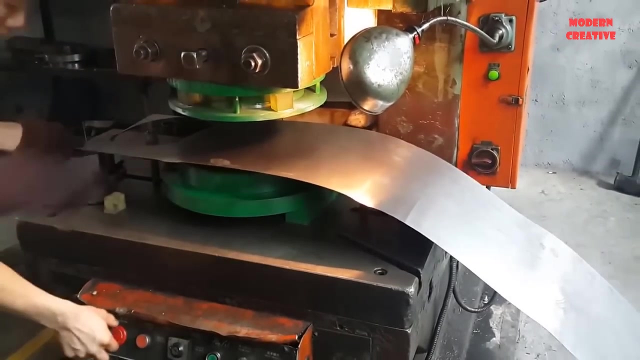 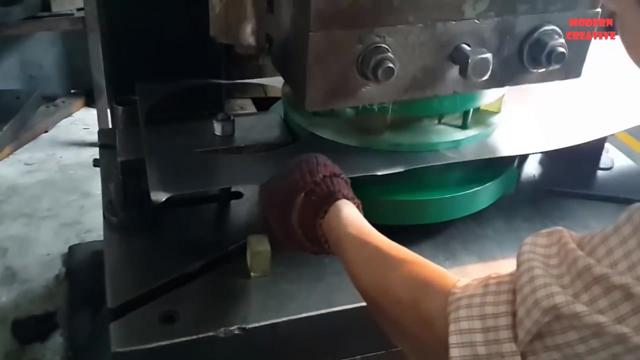 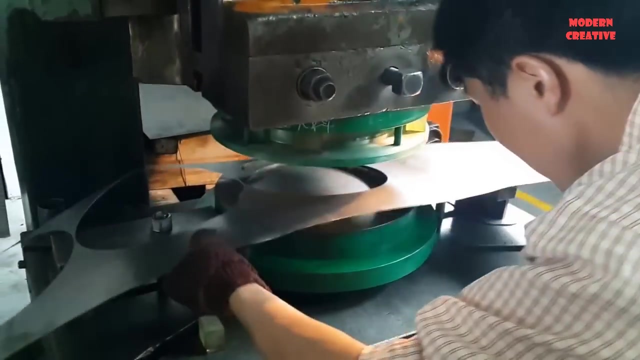 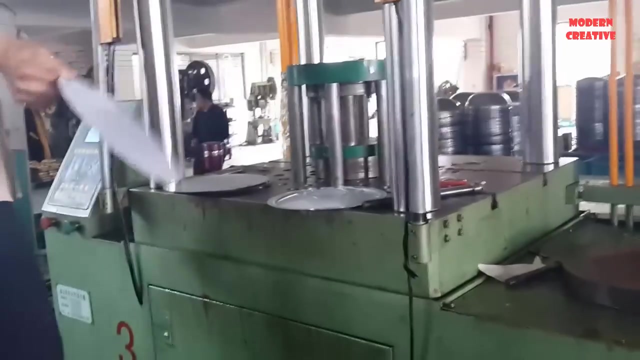 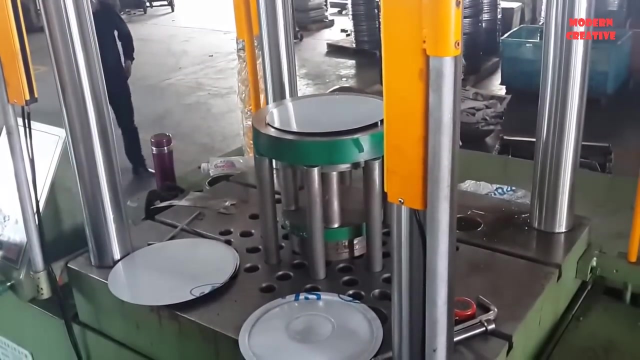 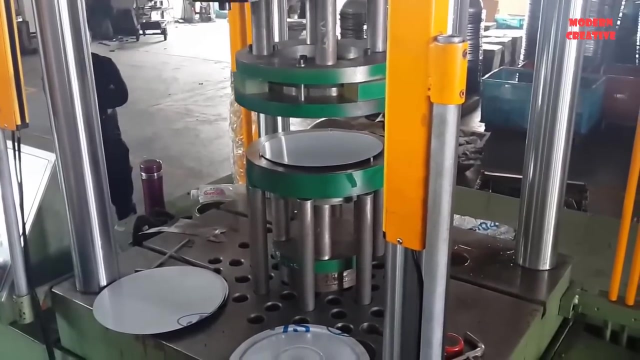 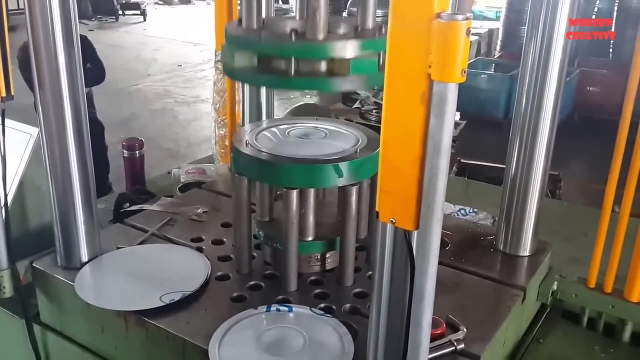 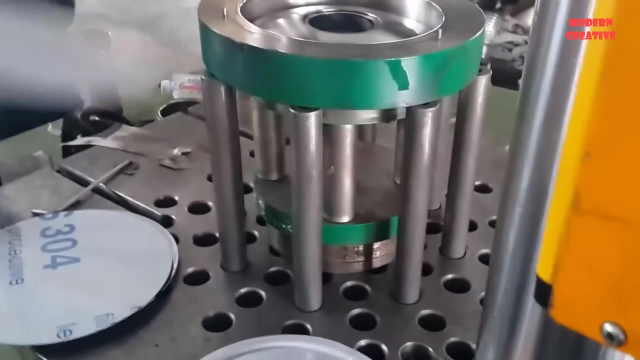 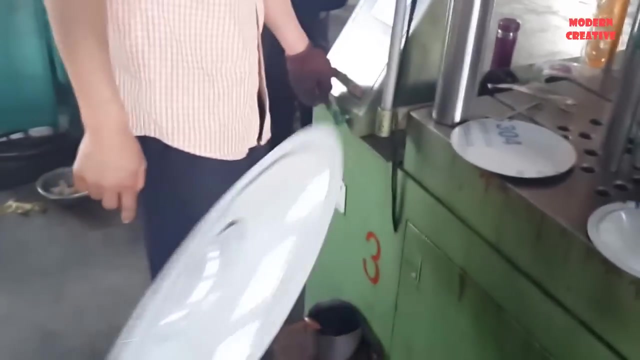 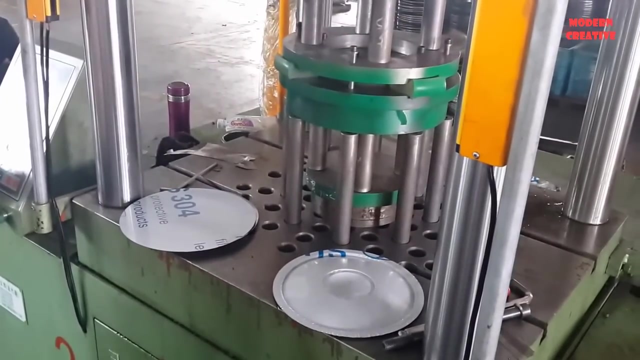 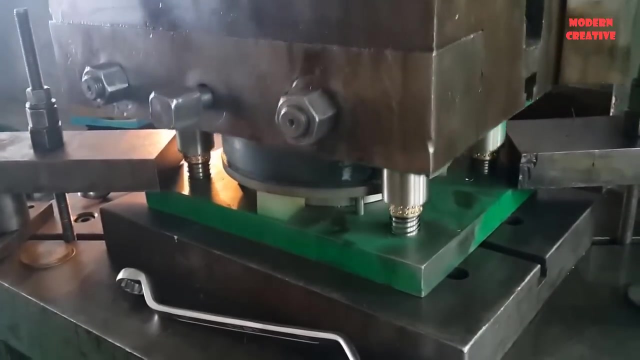 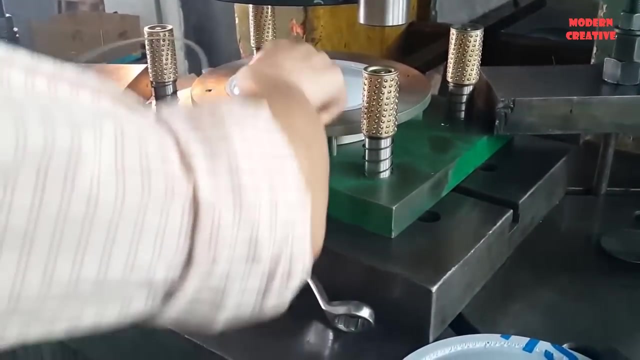 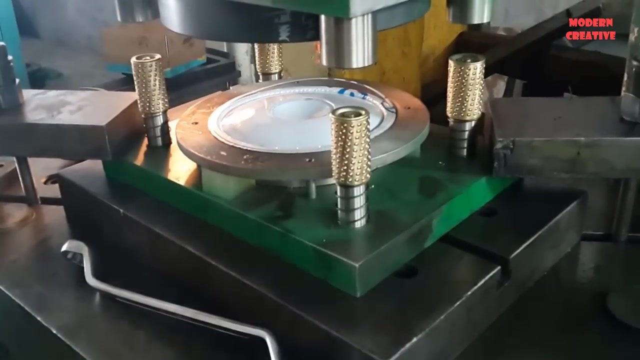 The front and rear of the head are molded to show the return shape. Thank you, Thank you. The hydraulic press is suitable for medium and heavy stamping in the manufacture of large parts and precision, among other applications. Thank you, Thank you.